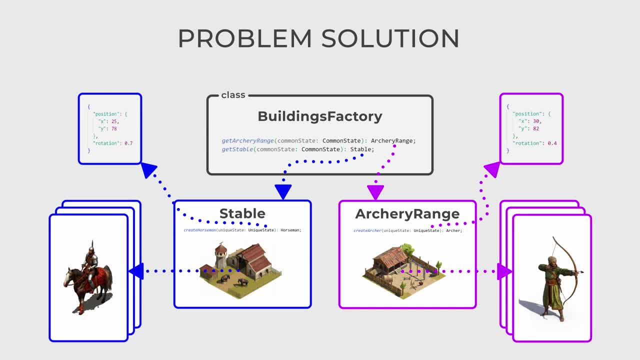 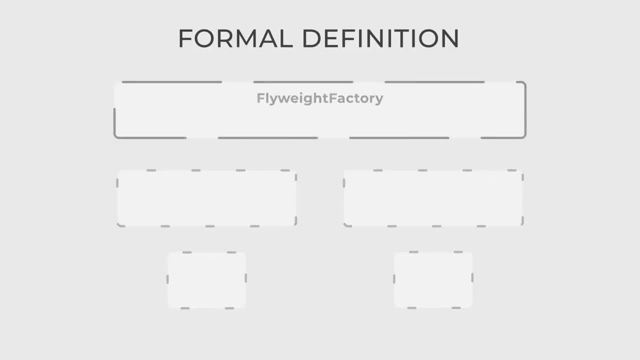 return new units to the client, ensuring that the units reuse their repeating state. There are three actors in this design pattern. First of all, FlyweightFactory. This is a class that contains methods for getting all available flyweight classes. The flyweight class is: 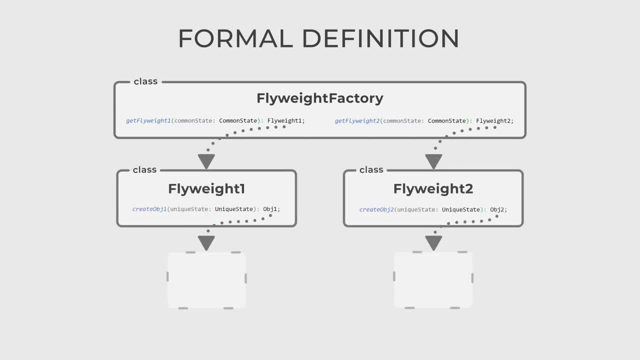 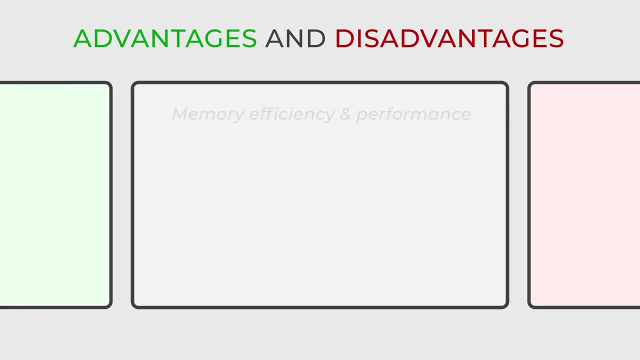 responsible for managing and creating flyweight objects. It ensures that the shared object state is reused And objects are the classes that flyweights creates and contain repetitive information that we are trying to optimize. On the positive side, flyweight is highly beneficial for improving. 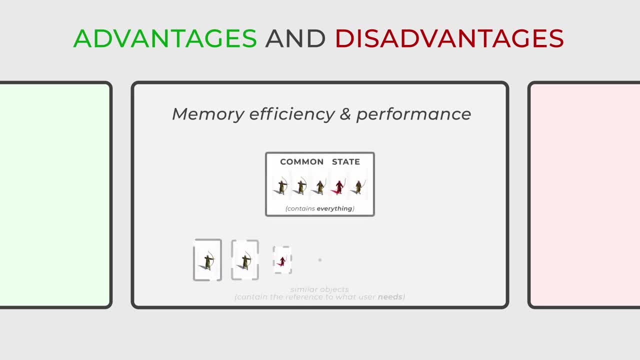 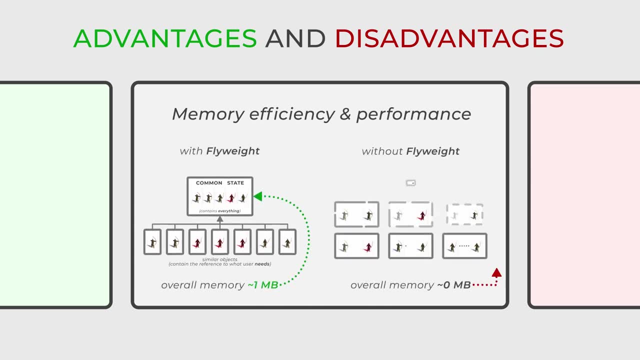 memory efficiency, as it enables the sharing of repetitive states across multiple objects, which is particularly useful when there are many instances of an object. This not only helps reduce memory consumption, but also enhances the application's performance by minimizing the over- and over-staffing. 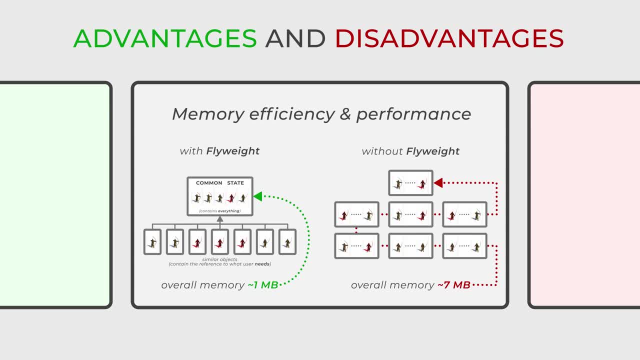 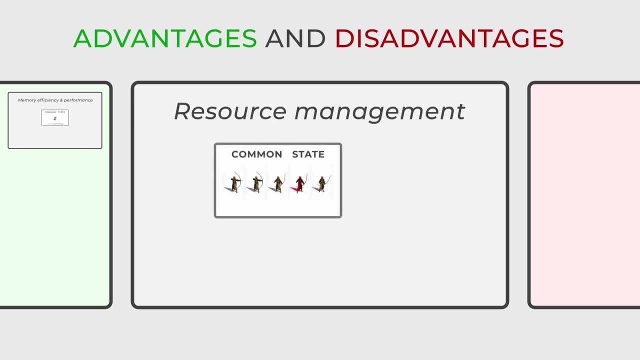 It also helps minimize the overhead associated with creating and destroying objects, especially in resource-intensive scenarios. Additionally, flyweight aids in resource management by centralizing the control and management of the lifecycle of shared objects, making it easier to handle them efficiently. However, there are also 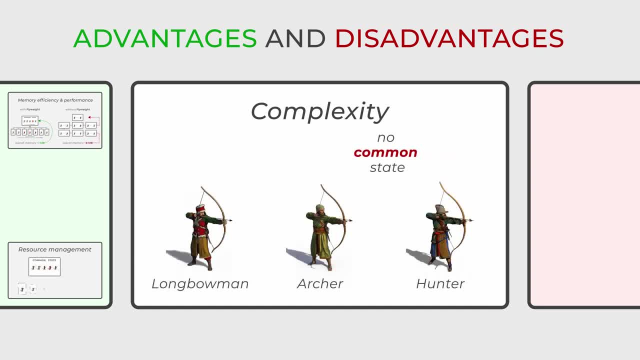 disadvantages to consider. The flyweight pattern can introduce a level of complexity, especially when managing extrinsic states that cannot be shared and need to be handled separately. This can make the implementation more challenging and lead to errors if not managed correctly. Additionally, because the flyweight pattern involves sharing intrinsic states among objects, 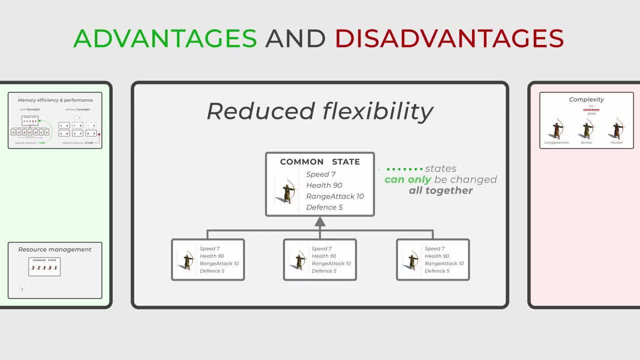 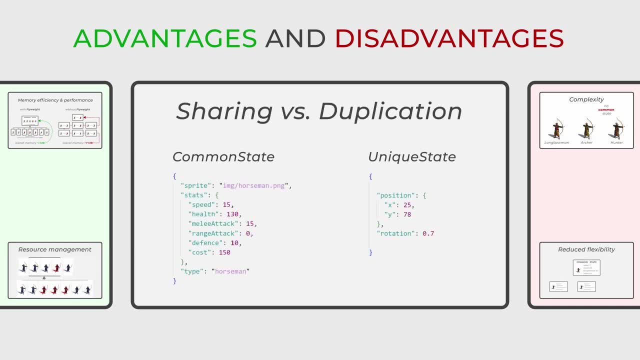 it might limit the extent to which individual objects can be customized, reducing flexibility in specific scenarios. Finally, there is a trade-off between sharing and duplication that needs to be carefully considered to ensure the correctness of the application, Deciding which states should be shared and which. 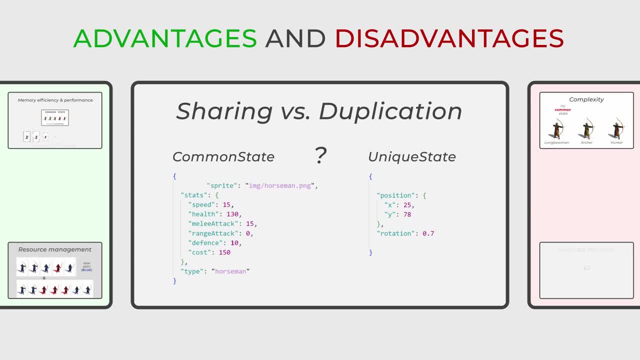 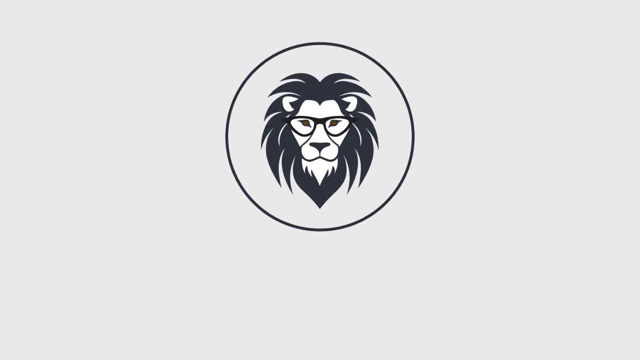 should remain separate, is critical to implementing the flyweight pattern. It requires serious evaluation to make the right choices for the specific use case. That's all about the flyweight design pattern. See you in the next video.